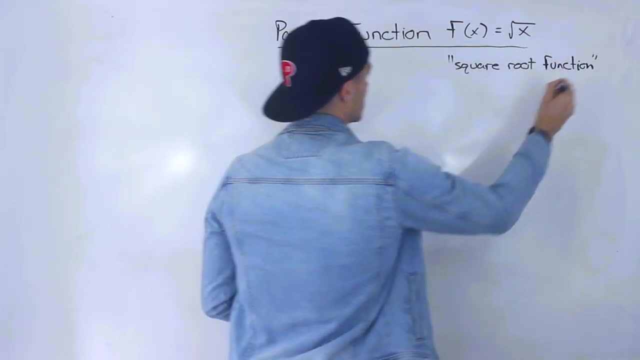 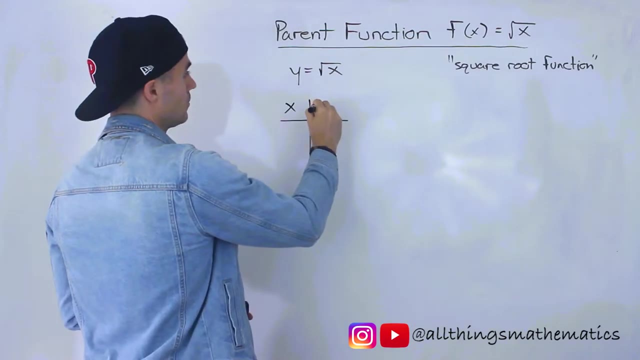 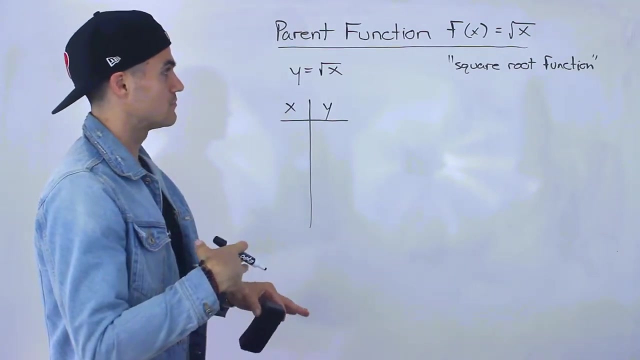 So let's make a table of values for this and see how it's going to look on a graph. Now notice that all of the x values they have to be greater than or equal to zero. Notice the x values can't be negative, because you can't square root a negative number. If you tried to take like 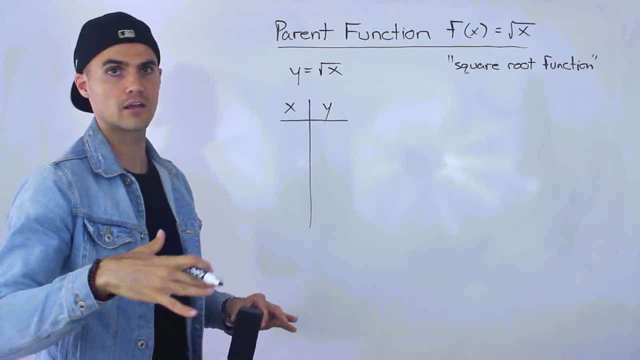 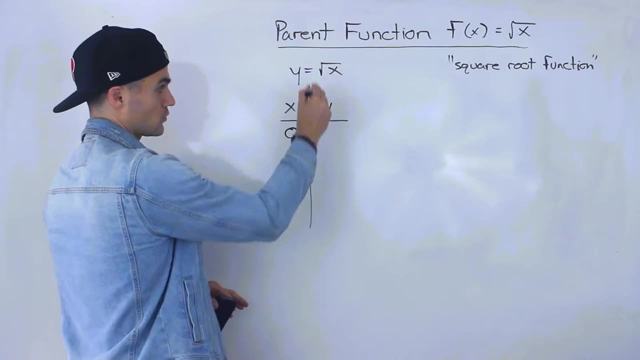 the square root of negative four. you'd get undefined in your calculator. So all the x values have to be greater than or equal to zero. They could equal zero, because the square root of zero is just going to be zero, And then the rest of the 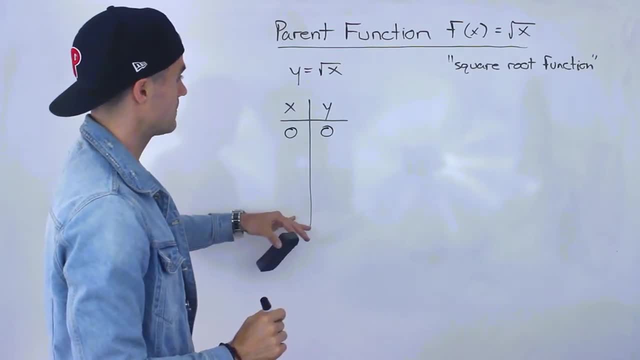 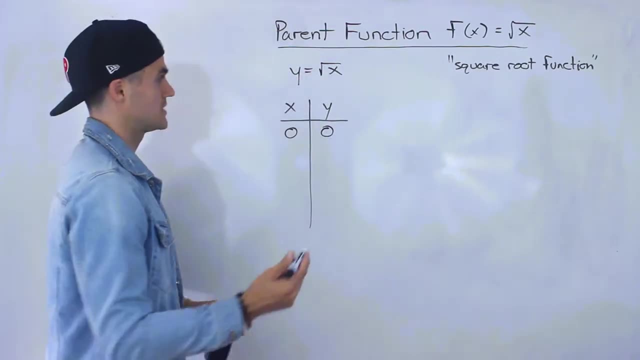 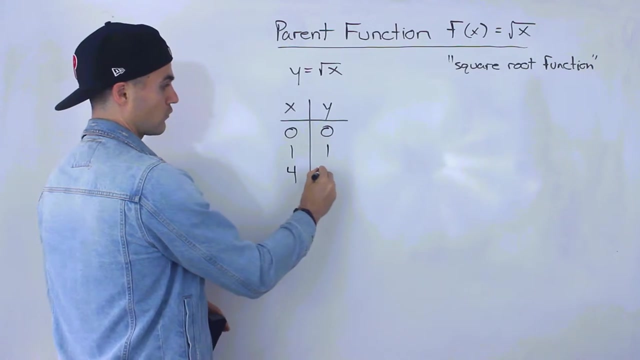 numbers have to be positive. So let's pick some x values here that make a smooth y value, meaning that when you square root them it's not going to be a decimal. So one would be one of them. Square root of one is just one. Another one would be four. Square root of four is two. 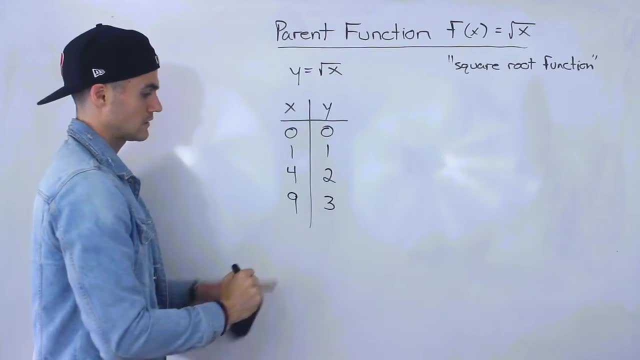 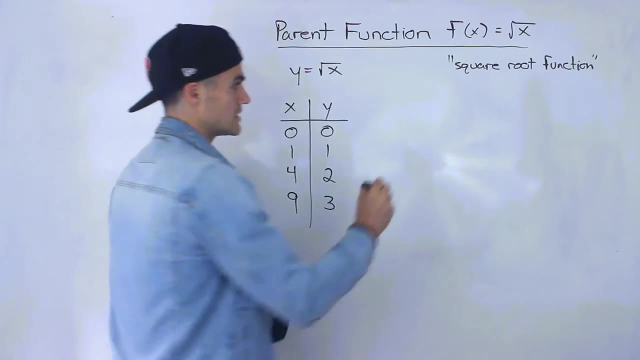 And then nine. Square root of nine is three. And then you could do 16,, 25,, 36, but let's cap it off at nine. So if we take these points and plot them, how's this going to look? So we're going to go all the way up to nine, So we'll have one. 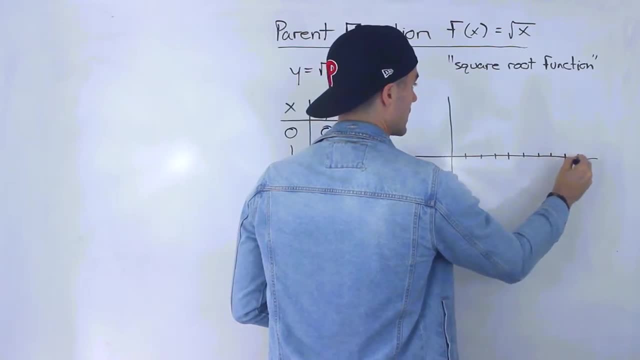 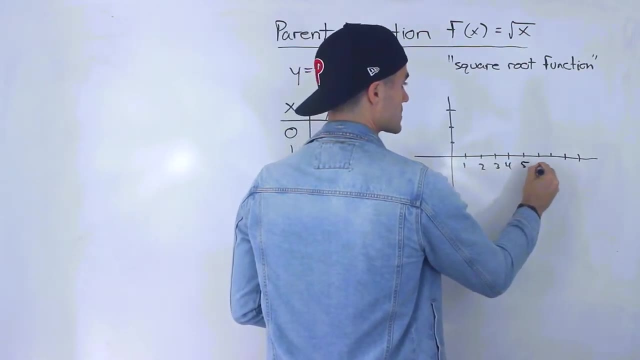 two, three, four, five, six, seven, eight, nine, And we'll have one, two, three. So we got one, two, three, four, five, six, seven, eight nine, And then one, two, three. it's easy to see there. 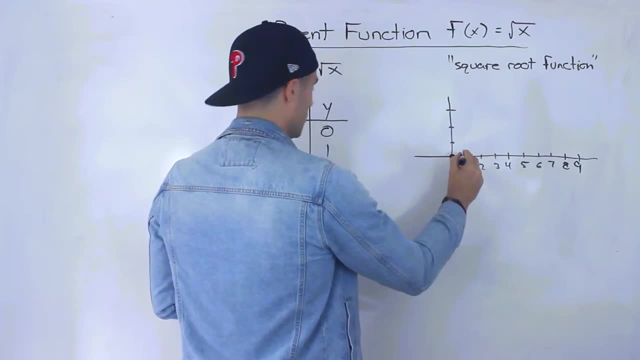 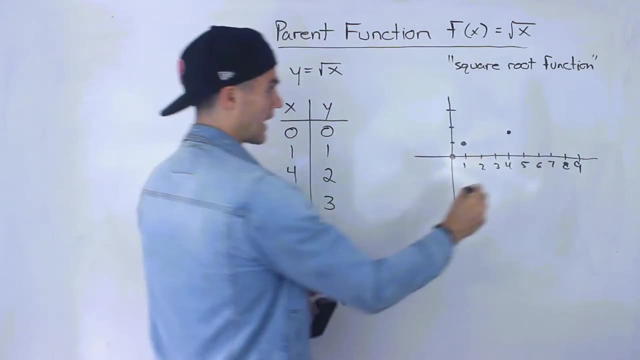 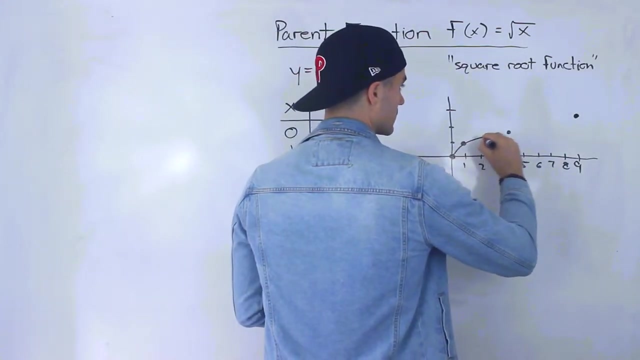 So we got zero and zero, We got one and one, We got four and two, which is here, And then we got nine and three, which is going to be over here. So if we connect all of these, this function is looking like that. 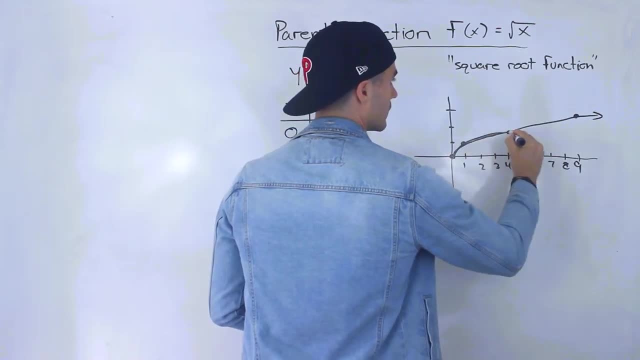 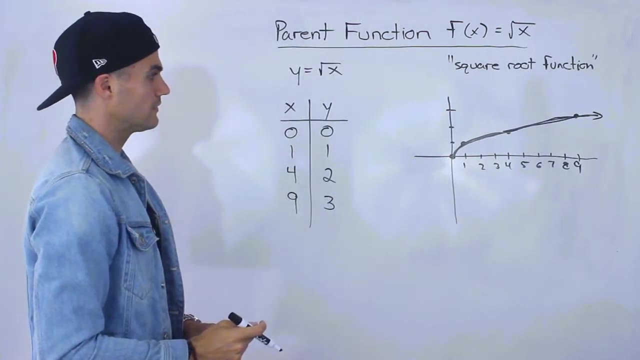 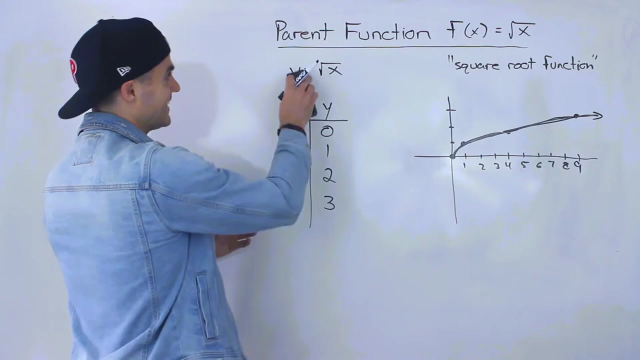 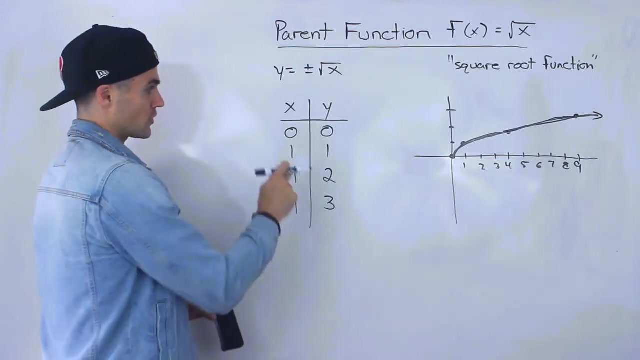 This should be more of a smooth curve here, But yeah, anyway, hopefully you see how that looks. Now, one thing I want to mention here is: notice that the square root of a number- technically it should be plus or minus, So, for example, the square root of one. 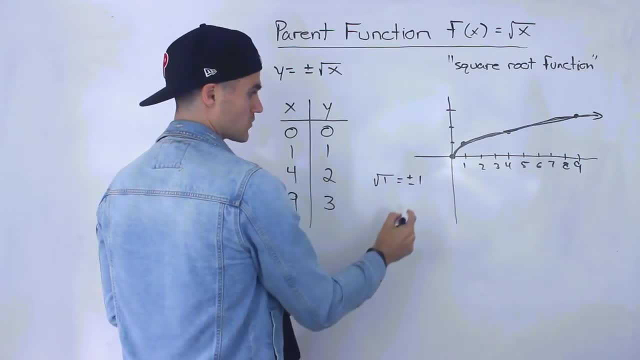 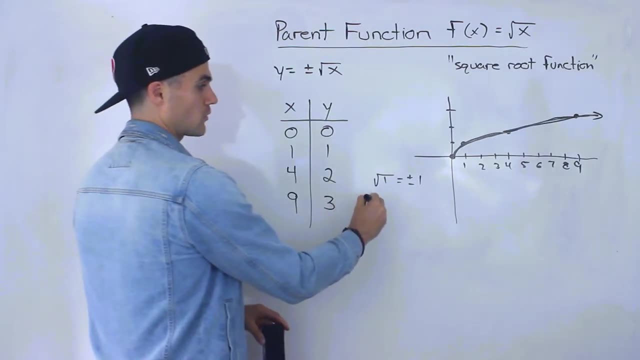 is technically plus or minus one, because one to the power of two gives us one and negative one to the power of two gives us one as well. Or the square root of four is plus or minus two. So why did we only put positives here? Because technically, 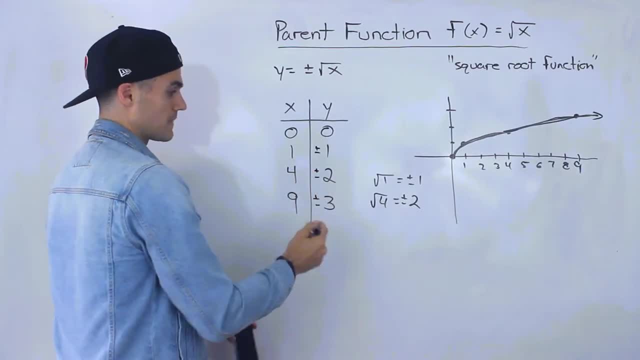 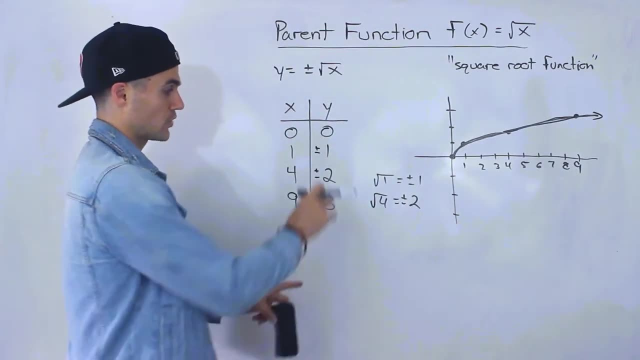 they could be plus or minus one, plus or minus two, plus or minus three, And if that happens, then we're going to have more points. We're going to have negative y values as well, And if we were to plot those corresponding negative y values, we'd have one and negative one, we'd have four. 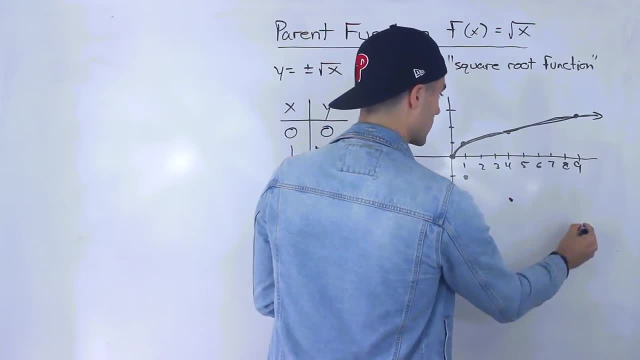 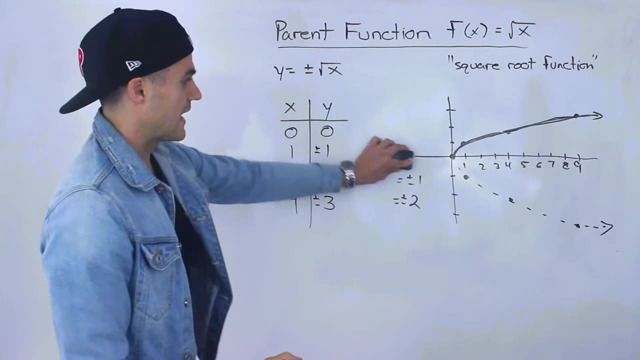 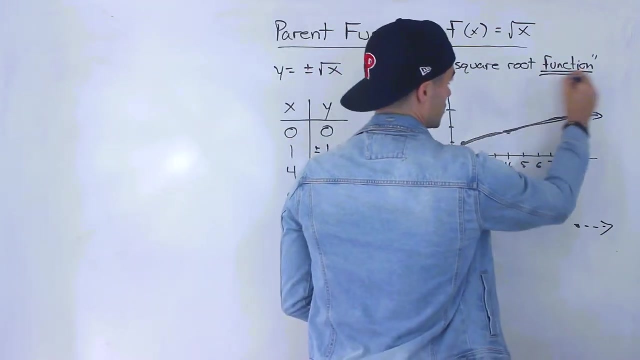 and negative two, then we'd have nine and negative three, And so there would be another part to this graph like this. The reason why we don't put the negatives is because this here we're calling it a function, We're calling it the square root function, It's a parent function, And so notice that if we were to 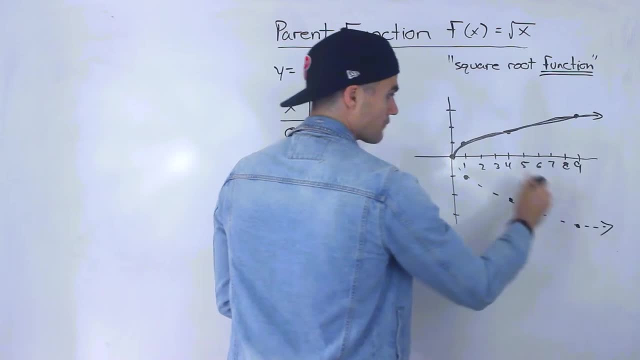 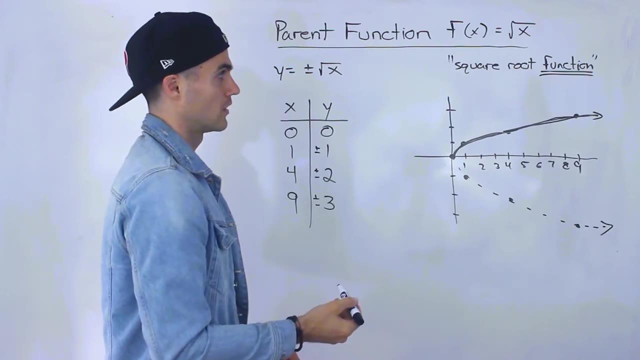 put the negatives here- and there was this other half of the graph- then notice it wouldn't pass the vertical line test, So it wouldn't be a function anymore. So when you're dealing with the parent function, the square root of x- 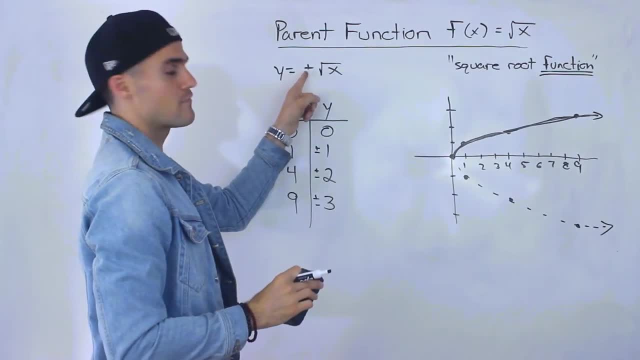 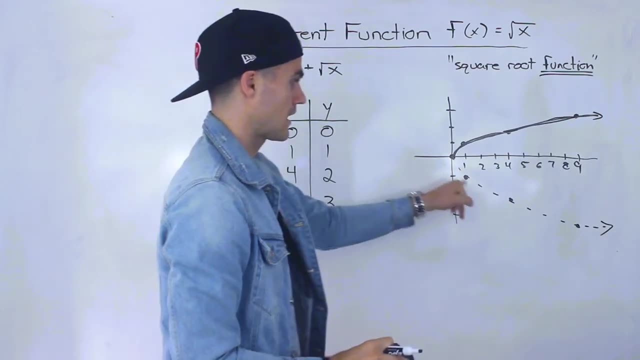 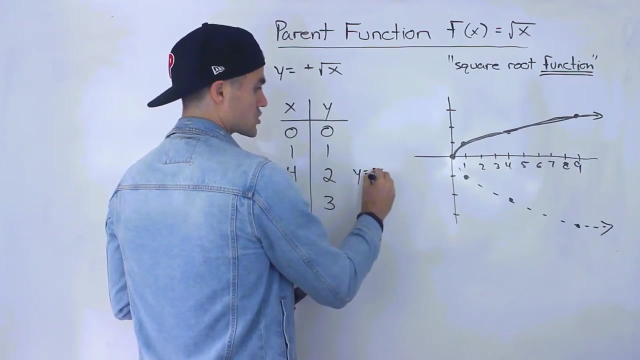 you're dealing with the positive y values, the positive square roots. Okay, so they would just be positive one, positive two, positive three, and we would ignore this part here. Now, one thing I want to mention is if you see y equals the square root of x, then you only deal with the positive. 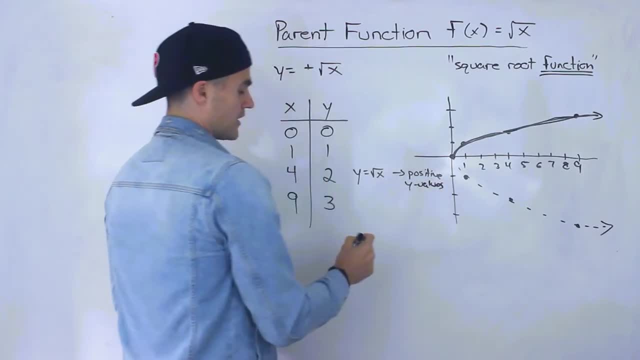 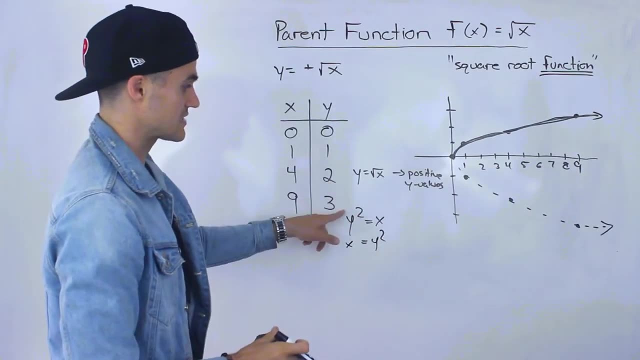 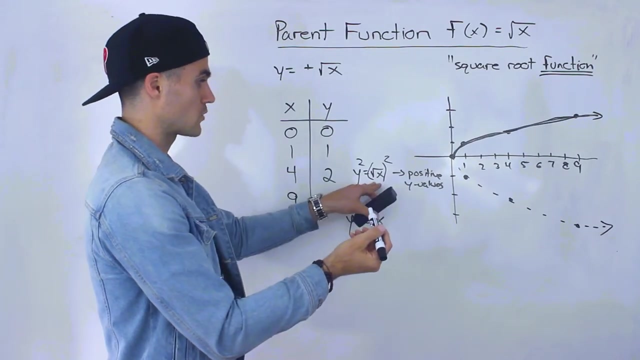 y values. But if you see something like y- y squared is equal to x or x equals y squared, Notice that this and this are the same thing. Basically, to get to here to here, we just squared both sides And the square root of x squared is x. 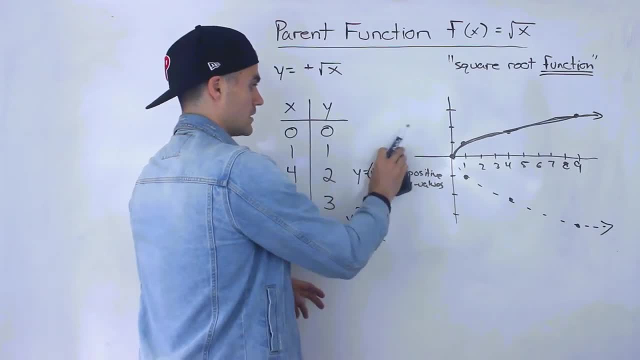 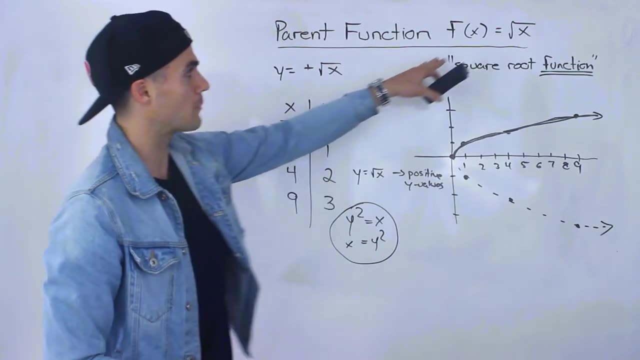 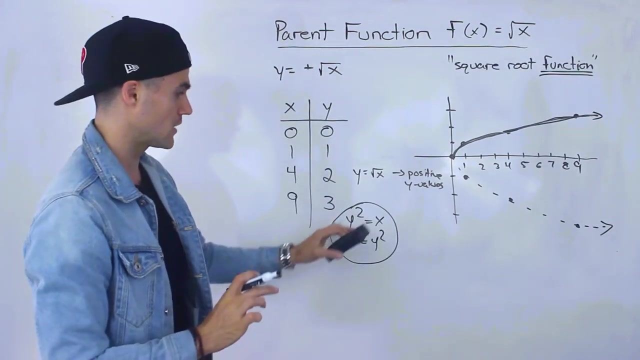 and then y squared is y squared here. So this here: if you see something in this format, it's not in that proper function format. function notation here: right, Because the y is not isolated. we got y squared equals x. If you see something like this, then you would deal with the